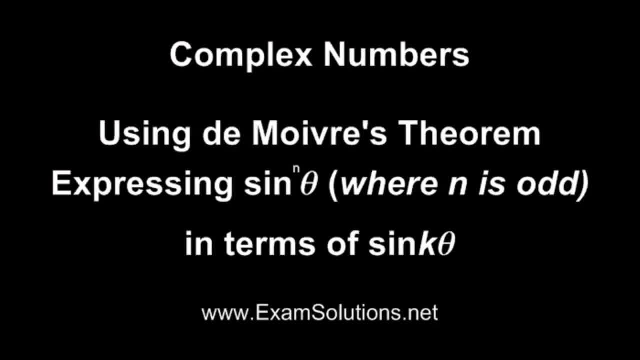 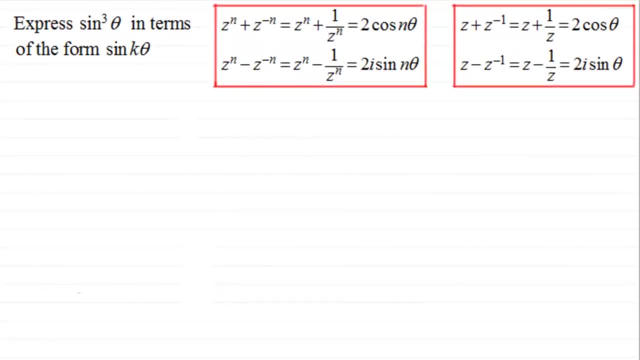 Hi, welcome to another video in my series of working with these identities. Now, in an earlier video, I showed you how we could use these two top identities to express powers of cos theta in terms of multiple angles. but in this video, what I want to do is show you how we can express sine theta in terms of multiple. 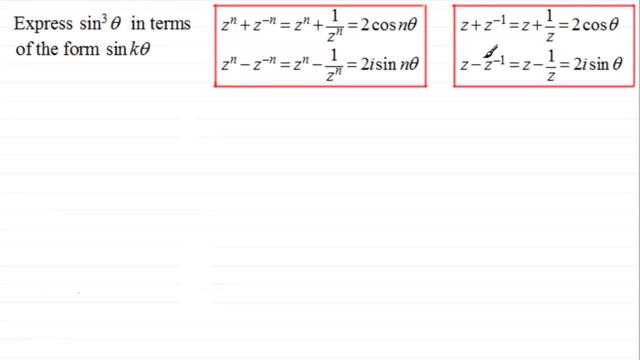 angles, and the example I'll use is sine cubed theta. We've got to express sine cubed theta in terms of the form, sine k theta, and you'll notice that the power here is an odd power and what I will show you holds for all odd powers. I'll 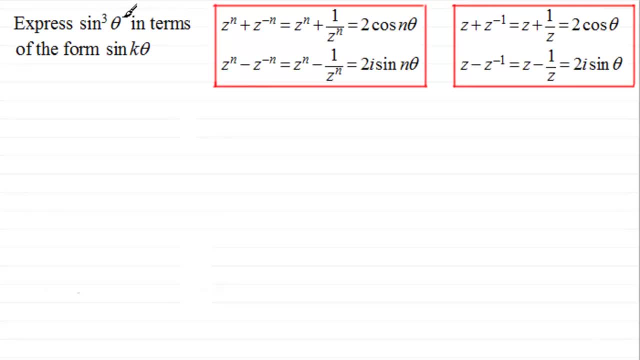 deal with even powers in the next video. Now, in the previous video we were looking at expanding cos theta to any power. ok, and we use these two top identities here. but when we're dealing with expanding sine theta to a given power, what we need to use is these two identities in the bottom here. So what? 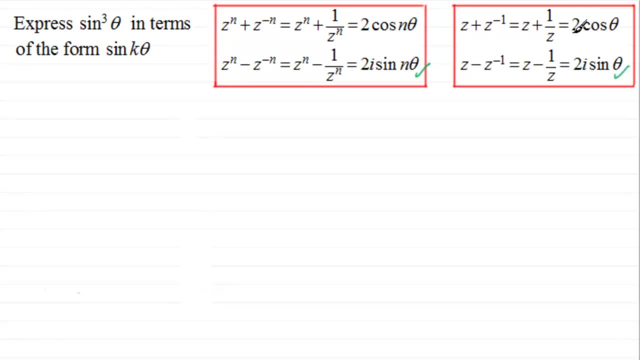 I'll do is I'll just simplify this, will remove the top two and just concentrate on the bottom two identities. So we have z to the power n minus z to the power minus n, which you could write as z to the power n minus 1 over z to the n is equal to 2i, sine n theta and in the special case, 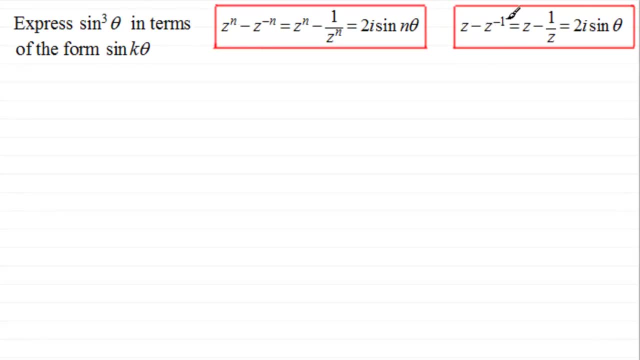 when n equals 1, we get z minus z to the power. minus 1 turns out to be equal to 2i, sine theta. So when we've got to express sine theta to any power, what we do is we take this identity here and we write 2i. 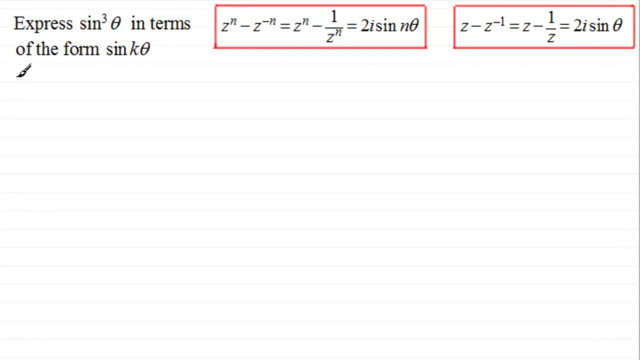 sine theta to whatever power we've got here. so we'll start off then just by putting 2i sine theta, and in this case it's all to the power 3.. So when we expand this, we will get sine cubed theta, so that's why we use this particular identity. now we know that this is the 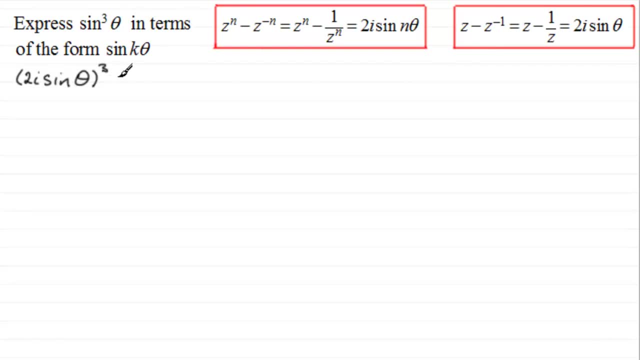 same as Z minus said to the power minus 1, so we can write this as being identical then to Z minus said to the power minus 1, all to the power 3, so whatever power you got here, just write this out to that power and then write Z. 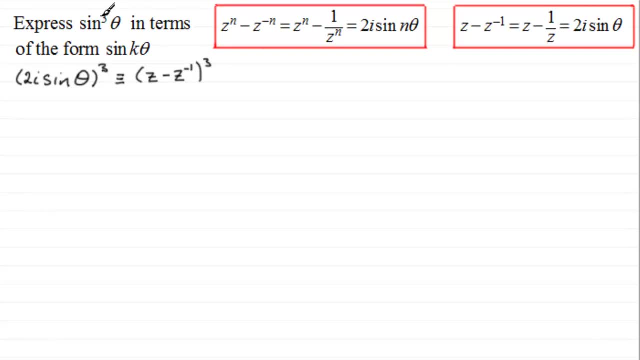 minus Z to the power, minus 1 to the power that you've got here. okay, now we need to expand the brackets and we do this, say, by using the binomial expansion formula, and in this example, we've got a, which is the Z, and the B is minus Z to. 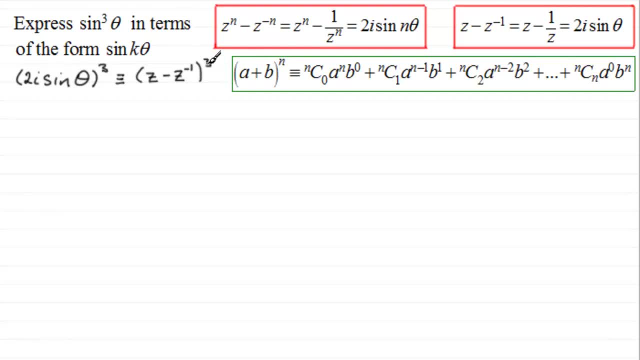 the power minus 1 and the N is the 3. so, working with this, you can write this as being identical to the power minus 1. so, whatever power you got here, just write this as being identical to the power minus 1 and the N is the 3. so, working with this, 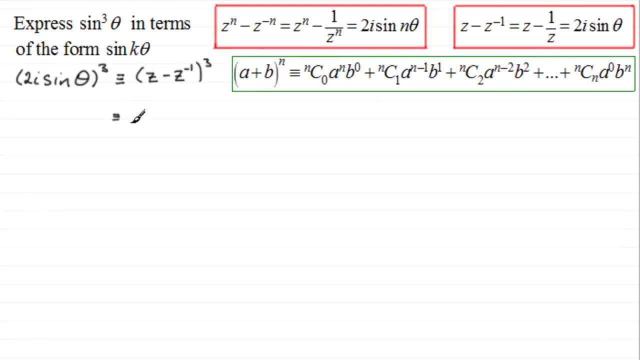 okay, expanding it in the usual way. we've got NC 0, so that's going to be 3, C 0. okay, multiplied by 8, the power ends, that said to the power 3, and then B to the power 0. so B, remember, is minus Z to the power, minus 1, and that is all raised to the 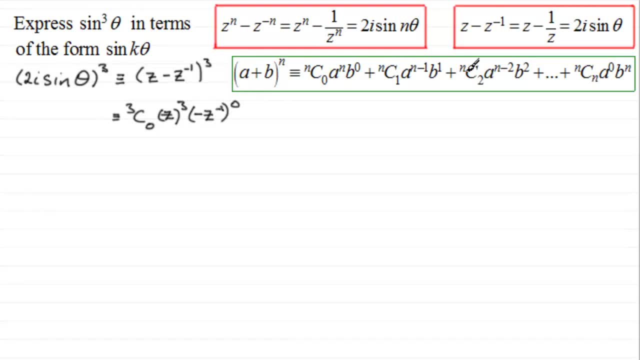 power: 0, and then we just work our way down for all the other terms. so we're going to have the following terms now, when we clean this up: okay, what we end up with is 3 C, 0 is 1, and you've just got Z cube. 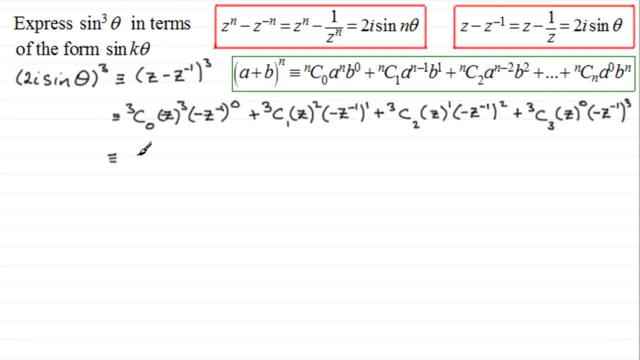 because minus Z to the power, minus 1, all to the power, 0 is 1. so you just got Z cube then for that first term, and then 3, C, 1 is 3 and then we've got Z squared times negative Z to the power minus 1. so just adding the powers gives us simply Z. so 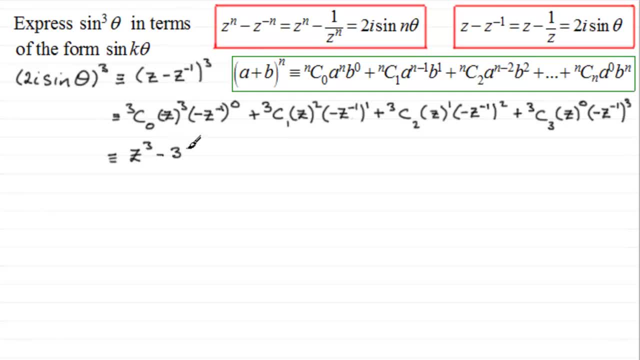 we end up with minus 3 Z for the next term, 3 C 2 is 3. so we're going to get a plus term here because you've got this minus Z to the power, minus 1 all squared. so you end up with plus 3 and then Z to the power, 1 times Z to the power. minus 2 is Z to the. 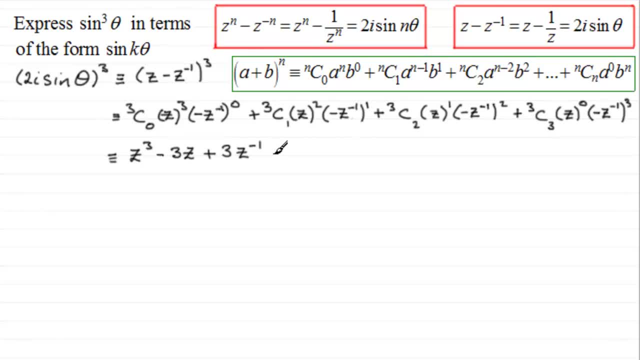 power minus 1. and then, on the last term, here you've got 3 C 3, which is 1 Z to the power. 0 is 1 a minus Z to the minus 1 is a negative value because you're cubing it and it. 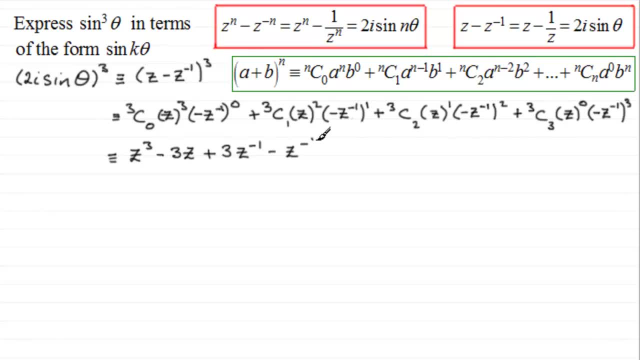 ends up being minus Z to the power, minus 3. now, what we do now is we group up terms in pairs that have this particular format. so that would mean that we we would group up the z cubed with the minus z to the power minus 3.. 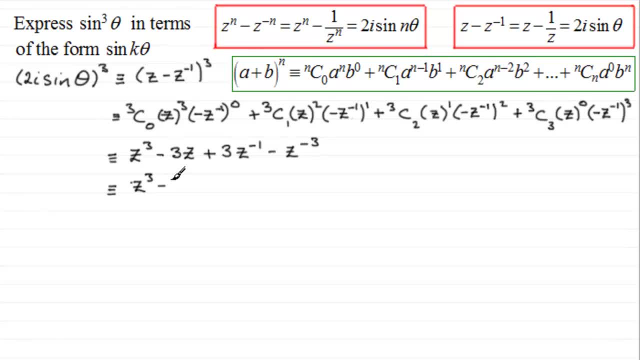 So z cubed minus z to the power minus 3.. Let's put that in brackets, not that you need to, but it does illustrate that pairing here, And then we can create that pairing again from these two, as long as we bring out the 3 as a common factor. 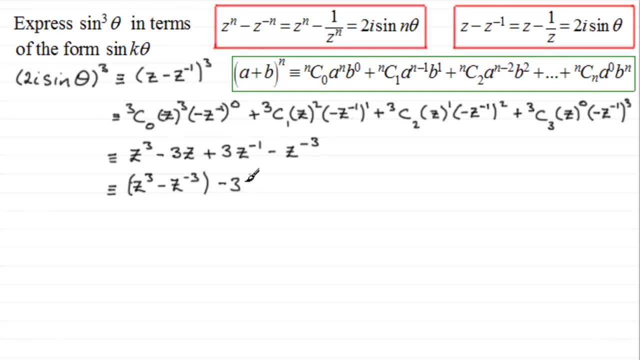 In fact, I'm going to bring out minus 3, so that we create z minus z to the power, minus 1.. OK, now, this should always happen with these types of questions. If you cannot get this pairing situation, then something's gone wrong. 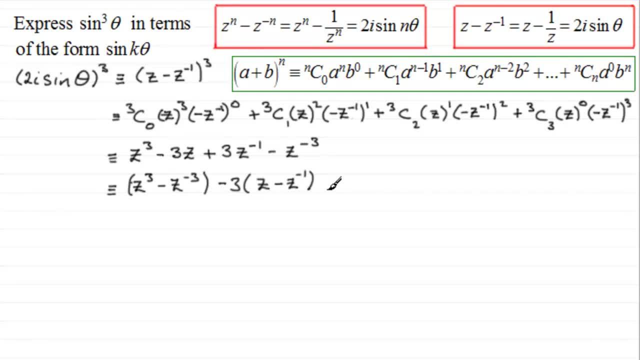 OK, so a valuable check when doing these kind of questions. Now we can pick up on what these values are: Z cubed minus Z. cubed minus z to the power minus 3. is this one here when n equals 3.. And it turns out to be 2i? then sine 3 theta. 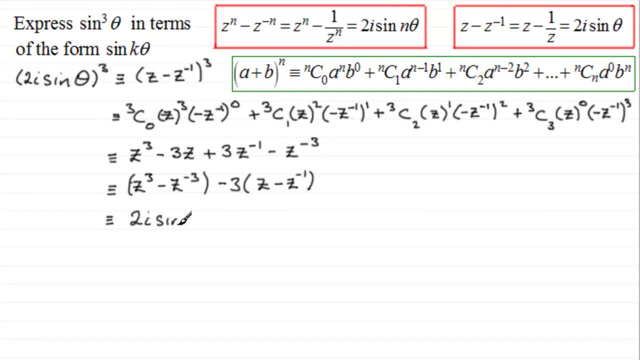 So just put here 2i sine 3 theta, And then for the next pairing we've got the minus 3, but z minus z to the power minus 1 is 2i sine theta. So we've got 3 times 2i sine theta. 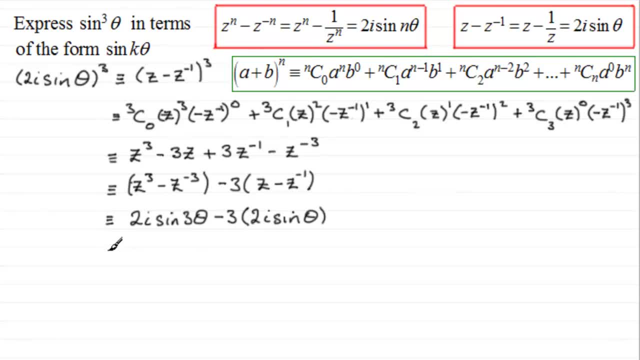 And if we clean this term up here, we've got that. this is identical then to the first term: 2i sine 3 theta. But on the second term we've got minus 6i sine theta. Now what we need to do is expand this bracket here. 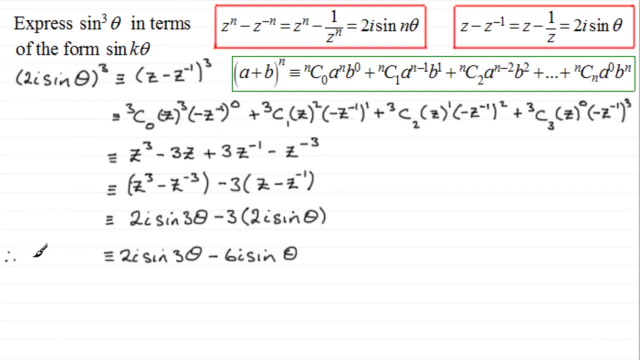 So, if I just take it down at this stage, here we've got 2 cubed, which is going to be 8.. We've got i cubed. Now i cubed is going to be minus i. So we've got minus 8i, and then we have, sine theta, all cubed. 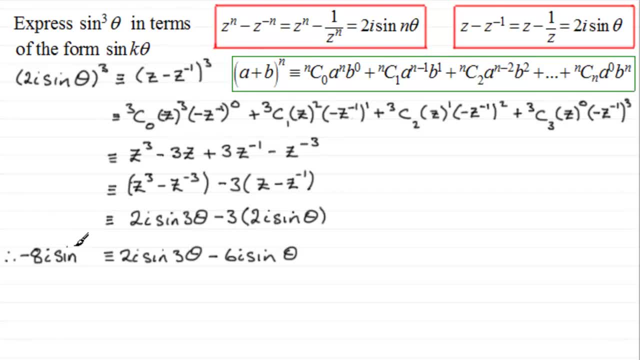 So we've got minus 8i sine cubed theta. So you can see that this term is imaginary and both these two terms are imaginary. So if we compare the imaginary terms, then we have got that. therefore, minus 8 sine cubed theta must be identical to 2 sine 3 theta, minus 6 sine theta. 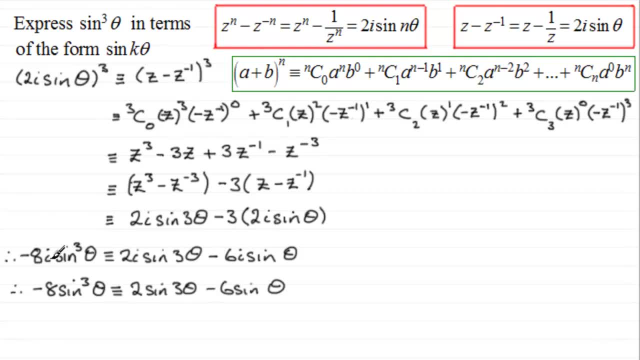 Okay, we can just strip off the i's on each term. Now we're asked to find sine cubed theta in terms of the form, sine k theta. So if we divide by minus 8, we've got that sine cubed theta must be identical to 2 divided by minus 8.. 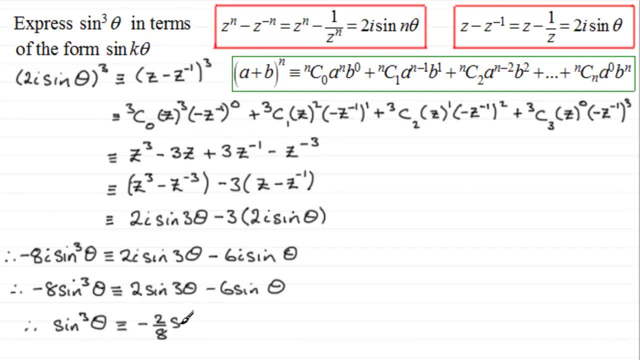 So minus 2 eighths sine 3 theta, And here we've got minus 6 divided by minus 8.. So it's going to be a plus 6 over 8 sine theta, And we can clean up these two fractions here. 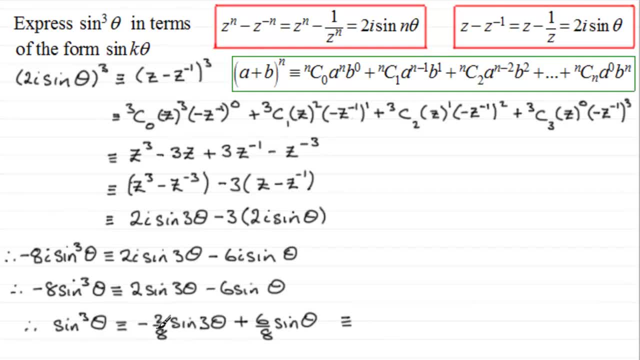 So we might as well say that this is identical. So we've got minus 2 eighths is minus a quarter. So you've got minus a quarter sine 3 theta. And then you've got 6 eighths, which is 3 quarters.